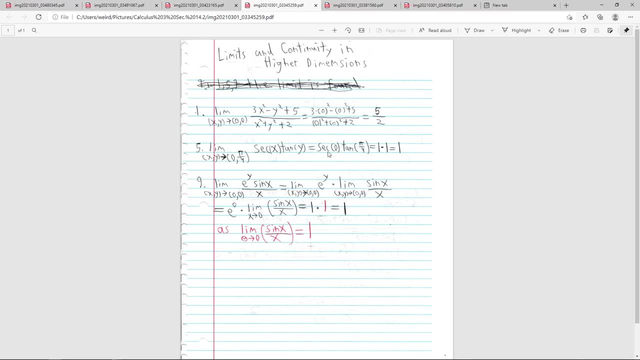 quite you know, quick, like that Number 5, it's, you know, approaching 0 and pi fourths, Secant x, tangent y, and we just plug in 0 and pi fourths And secant of 0 is 1.. That's because it's 1 divided by you. 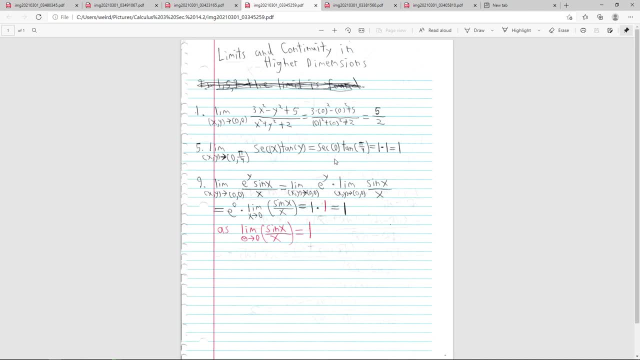 could think of 1 divided by cosine of 0 and cosine of 0 is 1.. So 1 divided by 1 is 1.. And tangent pi fourths similar: it's sine over cosine of those same values, Sine of pi. 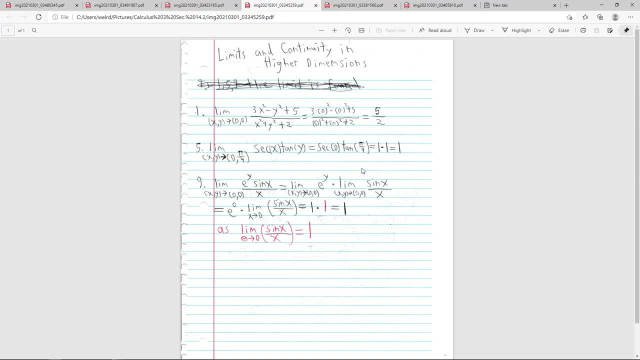 fourths is square root of 2 over 2.. Cosine of pi fourths is square root of 2 over 2.. So division by the same two exact numbers would be 1.. So it's 1 times 1, and that's. 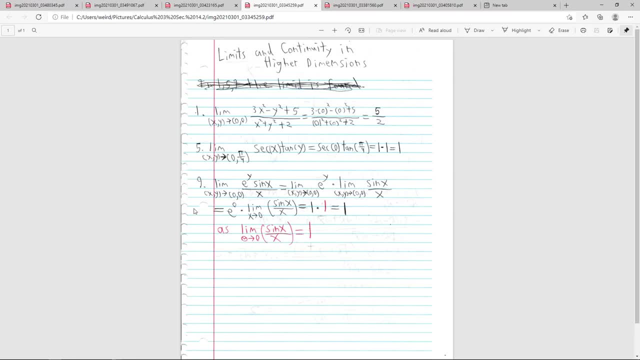 equal to 1.. Here's one where x and y approach 0, 0.. The limit is e to the y sine x divided by x. Now we have to actually make, do a little use, a little property, The limit of you know. 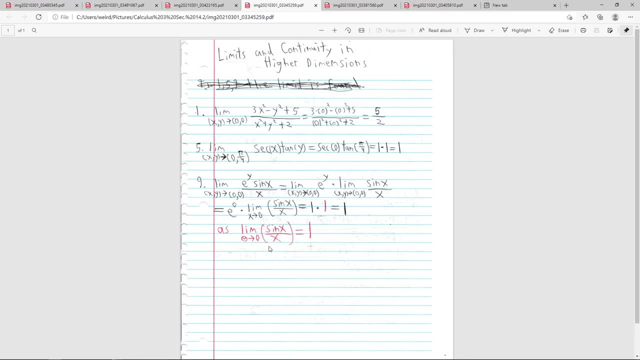 theta approaches 0 of sine. This should be theta and theta, But the point is: oh, you can say x approaches 0. Either one. that's a little mistake, but I'm trying to use a general example, I guess. 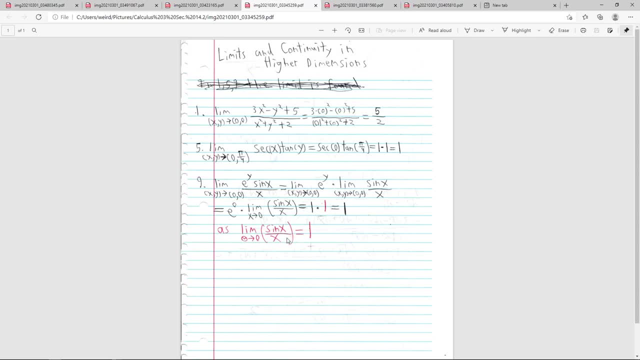 Same thing, Basically the limit, as you approach it, of you know this expression of sine x over x, of x approaches 0, or theta approaches 0,, or whatever you want to do with the variable of sine, So sine of theta, or sine of x over x over theta. whichever variable, same variable. 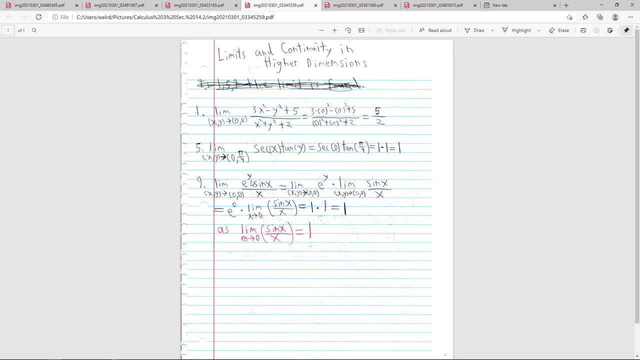 point is it's equal to 1.. And we can. this is multiplication, so we can split it up into two limits. You know, limit of x, y approaches 0, 0.. e to the y times. limit of x, y approaches 0, 0 of sine x, x over x, And that's e to 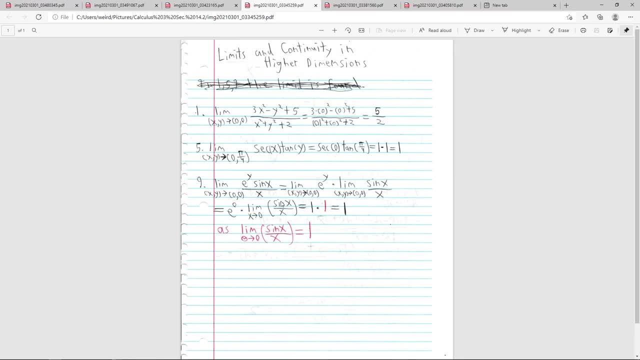 the 0, you know you evaluate it 0 times and this can be simplified down to just x, because that's the only variable present, in that x approaches 0 of sine x, x which is equal to 1 times 1, because e to the 0 is 1, and that's. 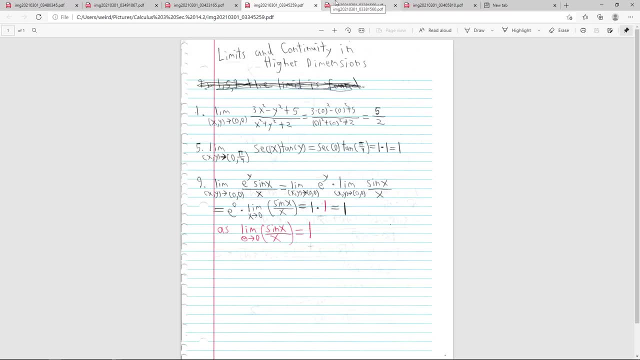 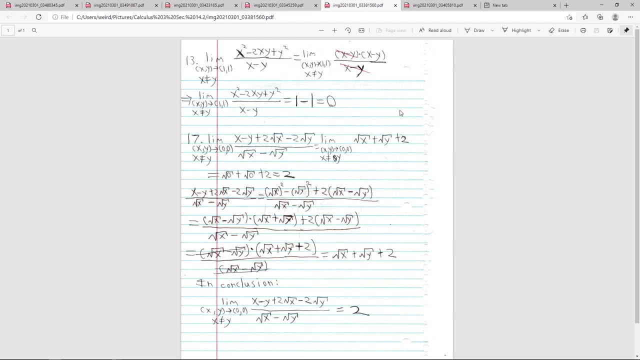 1. So it's equal to 1, again like the first bomb. Okay, time for a little bit more tricky. I think Now we have to use a trick where we simplify the expression before we can evaluate it. So x squared minus 2xy plus y squared divided by x minus y. 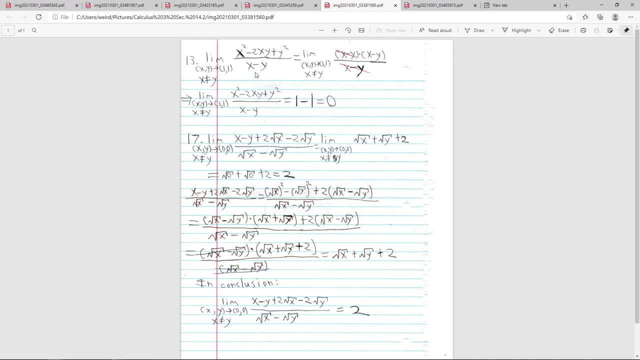 x, y approaches 1, 1.. So if these basically approach each other, 1 minus 1 will eventually equal 0, and that can't exist in the denominator, so we have to eliminate it, And we do this by factoring this into two binomials. 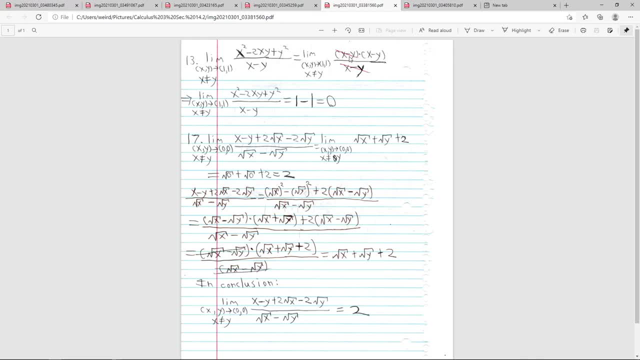 I think that's a good idea. x minus y, it's x minus y squared, because I think it's a difference of squares or whatever I think technically. Regardless, if you figure it out, it's x minus y times x minus y divided by x minus y. 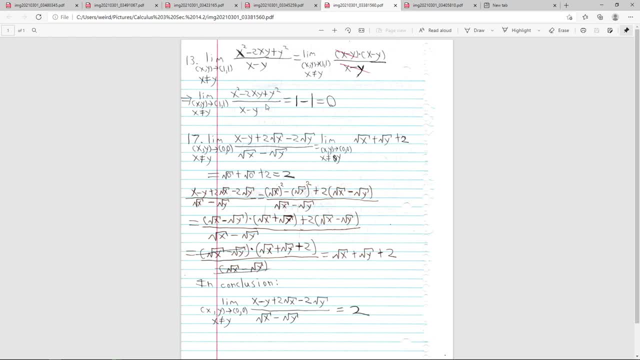 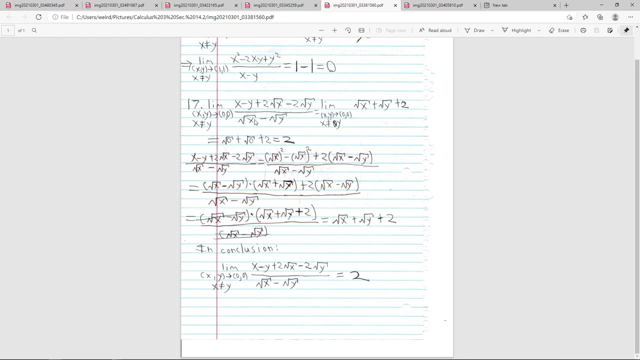 So it just becomes x minus y, You know, and x minus y is 1 minus 1.. So it's equal to 0.. Um, This one, this one's a little bit more complicated. It's approaching 0,, 0,, and square root of x minus square root of y is in the denominator. 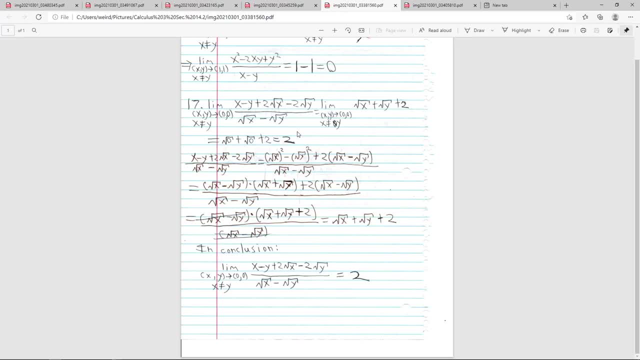 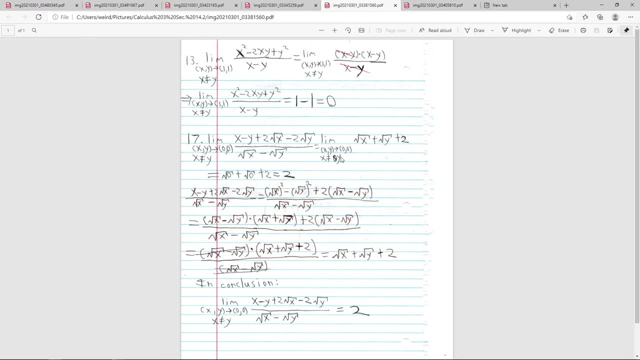 So that means it would be 0 minus 0, so you have 0 in the denominator. Okay, we have to get rid of that. we have to eliminate that stuff in the denominator. So this is equal to: oh yeah, and I skipped the works down here, but this is basically. 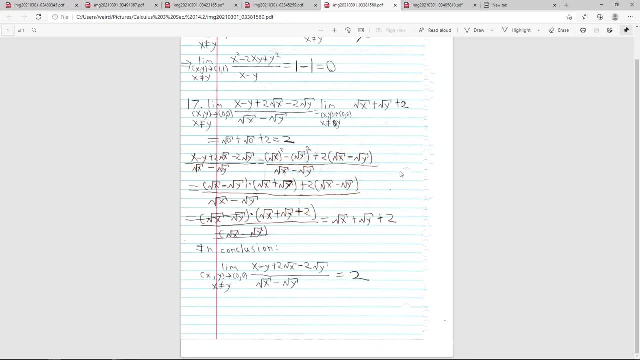 we end up with. we're going to end up with that at the end. I basically showed this, so I don't have to repeat writing out that limit, because these limits are kind of annoying to repeat, especially when you have multiple variables. it gets. 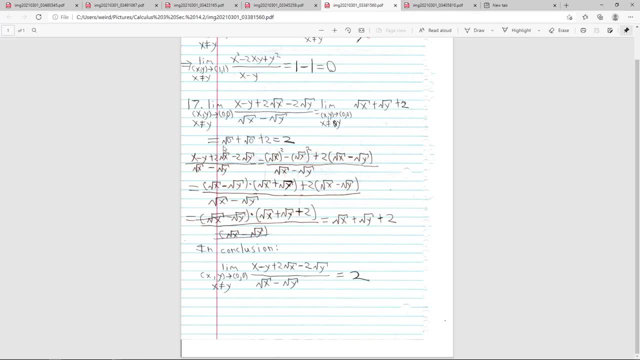 really complicated. it gets a lot of space, a lot of small spacing. So we're simplifying this expression. I copied down just the expression itself, but how we could, in any type of algebraic expression, simplify it. So: square root of x squared minus, square root of y squared plus yeah, so I basically converted. 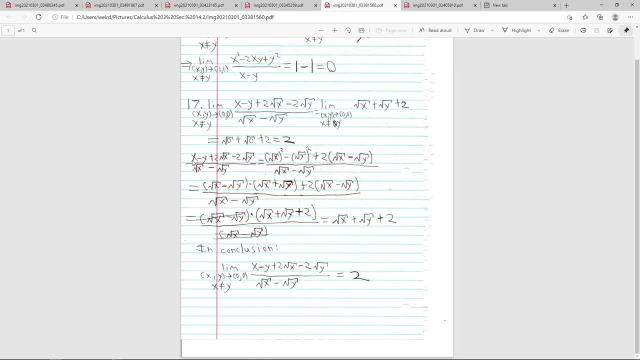 x minus y, like x and y themselves. Okay, Square root of them, but squared, you know it's the same expression, because the square root of something that is squared will be the number inside. So x is equal to square root of x squared, and y is equal to square root of y squared. 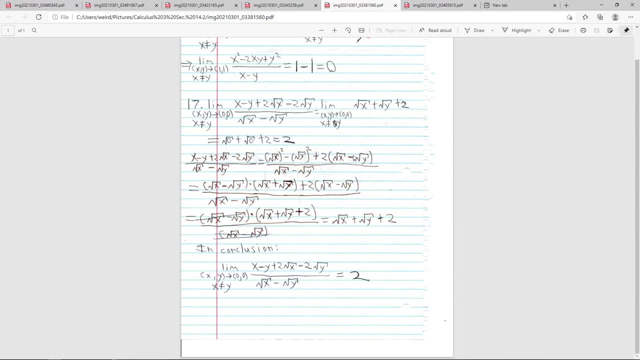 And I also distributed out a 2 from square root of x, you know, square root of x minus 2 square root of y to make it, and there'll be a reason for that in a step. So we we turn this into 2.. 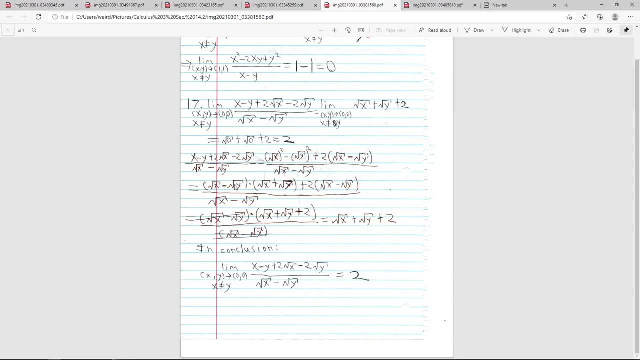 We basically factor it out. do factoring the difference? it's basically a difference of perfect squares- I guess you could say so using the technique- and it's square root of x minus square root of y times. square root of x plus square root of y is what you get. 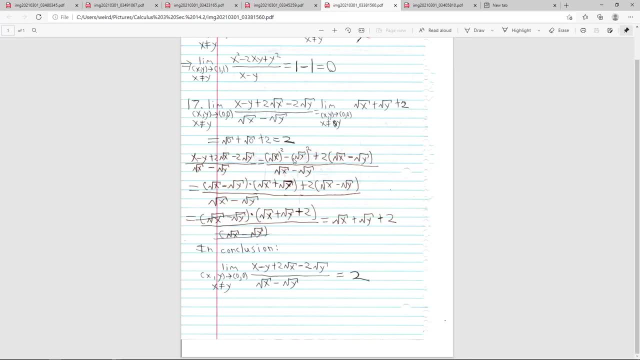 from this first part. The denominator hasn't changed yet. we're trying to eliminate the denominator somehow, And then you, it's this, hasn't? we still have that distributed out. The point is that square root of x minus square root of y and square root of x minus square 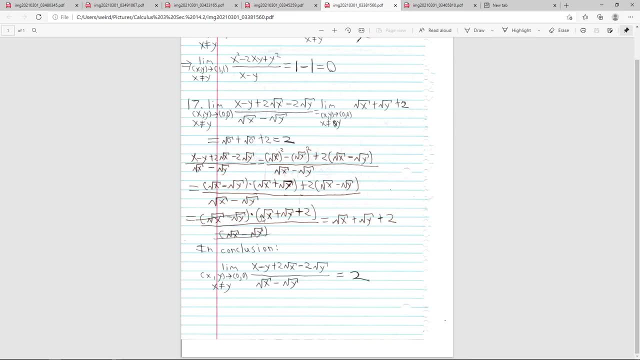 root of y are both in both expressions. so you distribute that out of the whole thing and get square root of x plus square root of y plus 2 from this And you cancel out the denominator and you get square root of x plus square root of y. 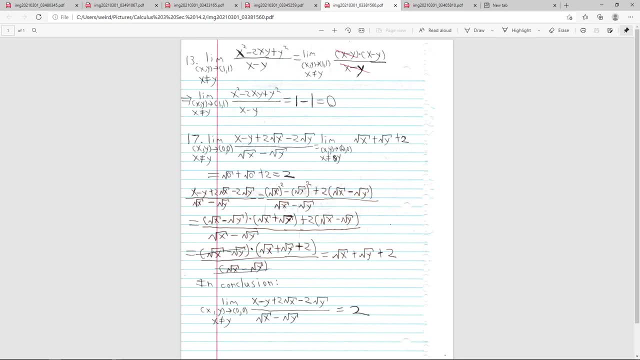 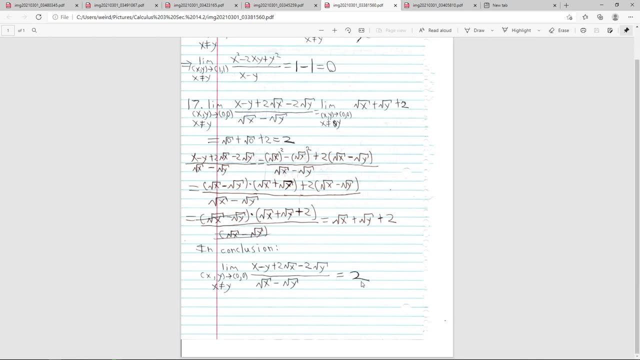 plus 2.. That's what's up here. That's where we evaluate the limit at, you know. so it's square root of 0 plus square root of 0 plus 2, which is equal to 2.. So the whole limit's just equal to 2.. 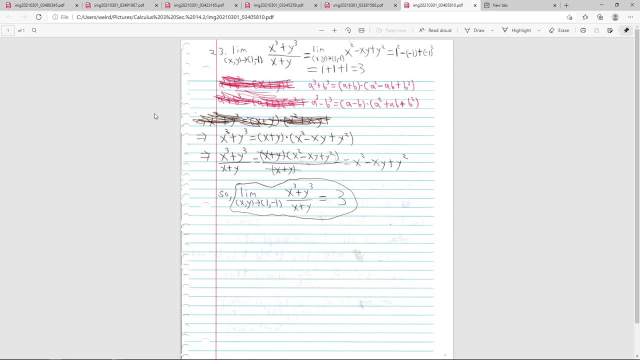 So this one, another evaluation, this one's not that bad if you, but you have to really recall this trick: A cubed plus b cubed, then a cubed minus b cubed. can be factored, these expressions: First one a plus b times a squared minus ab plus b squared, and our one is a minus. 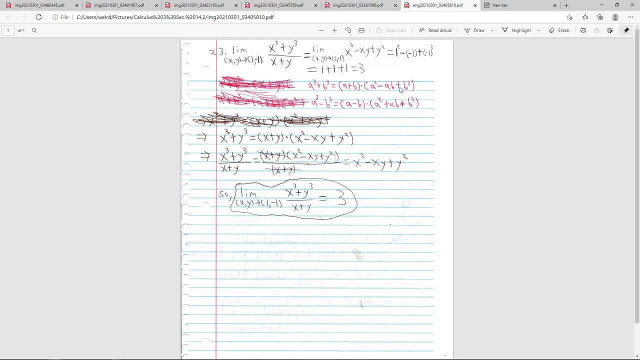 b times a squared plus ab plus b squared. So this sign stays the same. you can remember it. And this one's the same as that expression. This one's always positive. the last one, First one, is the same as the sum or difference. it's the same. then this one is the opposite. 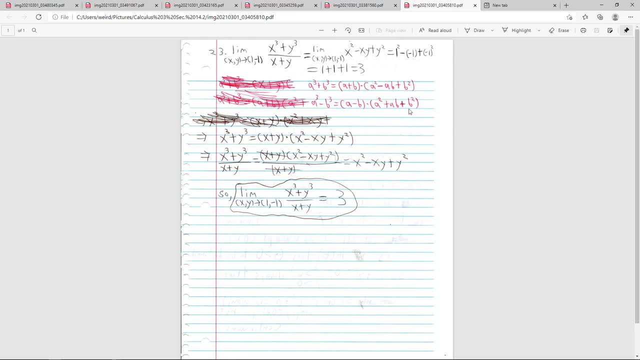 So plus minus, plus, minus, plus, plus. You know, so it stays. you know, I think SOAP is an acronym, You could say so it's same. so same sign, opposite sign and then always positive sign. That's how you factored us. 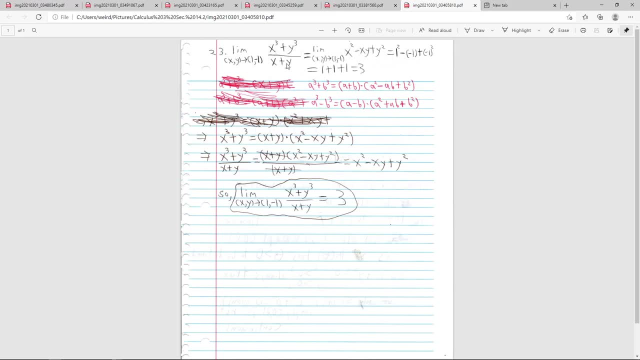 And you have to use that because we have to eliminate. we have x cubed plus y cubed divided by x plus y. So down here again, like last time, this is equal to x plus y times x squared minus x, y plus y squared, basically divided by x plus y. 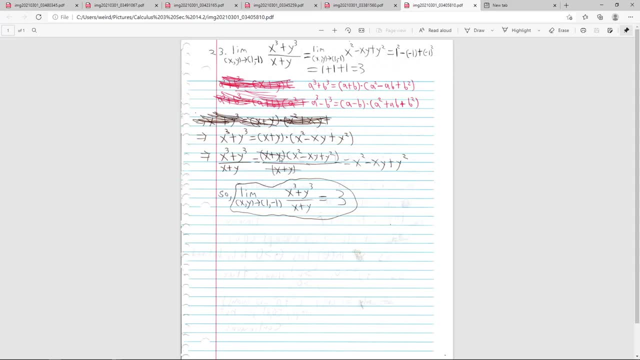 You know, I'm applying it very quick and it becomes just x squared minus x, y plus y squared. So that's where we evaluate the limit as it approaches 1, 1.. Oh, no, 1, negative 1, yeah, so it's 1 squared minus negative 1 plus negative 1 squared. 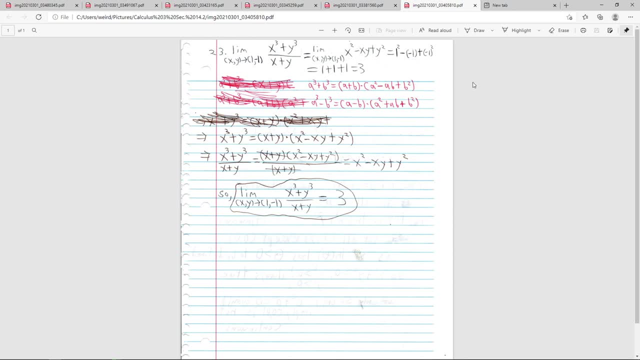 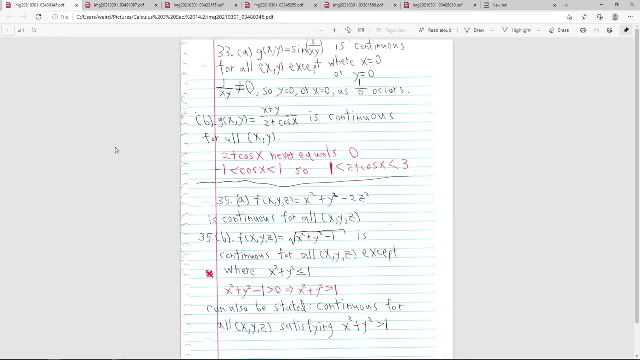 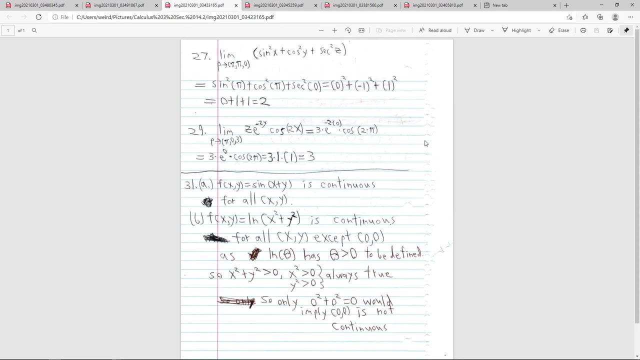 is what it's down to, and plugged in, It becomes 1 plus 1 plus 1 equals 3, so you okay. So finally, we just have to look at some continuity problems where you just tell: if it's continuous, We do it. yeah, oh wait, no, we have a couple more limits. 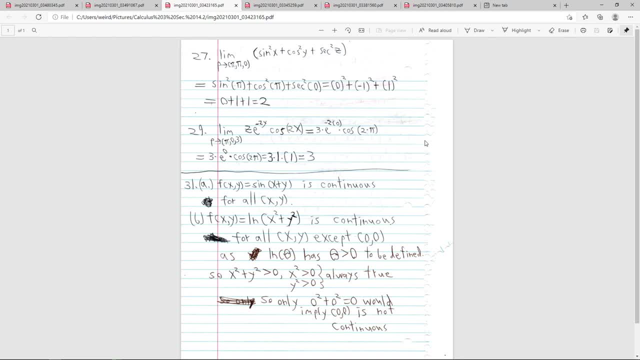 So these ones, we don't have to do anything, we just have to plug in. pretty much No cancellation for these last couple. So yeah, p is used commonly for three variables, so sine squared x plus cosine squared y plus secant squared z. 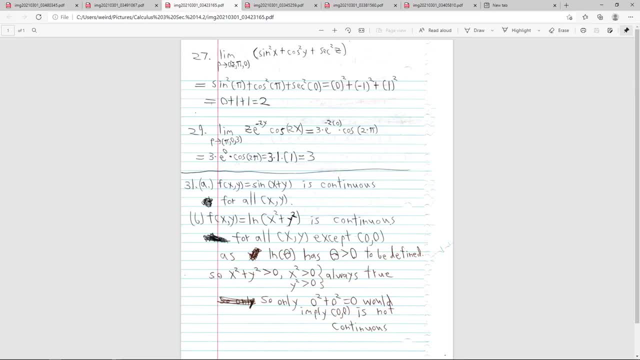 Pi, pi, Pi and zero. we plug in respectively. So sine squared pi plus cosine squared pi plus secant squared zero. So this is just sine cosine and secant values squared, So zero, negative 1, and 1, because sine of pi is zero, cosine of pi is negative 1, and 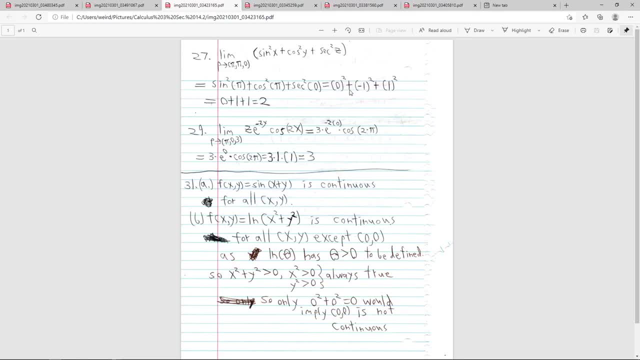 secant of zero is, as I said before, it's 1 divided by 1, which is 1.. You square each of these values so you get zero plus 1 plus 1.. That equals 2.. That's what the answer is. 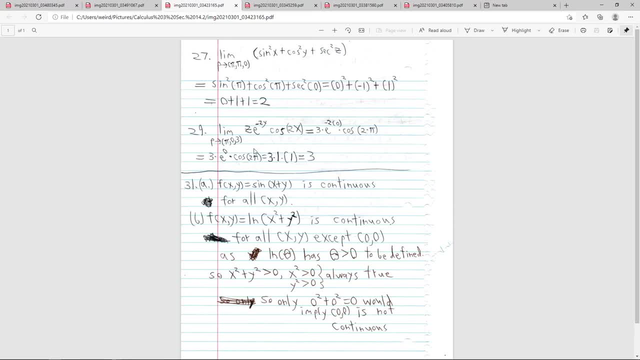 Then this one is z e to the negative 2y, cosine 2x, and we have to evaluate it. pi zero is 3.. So that's 3 times e to the negative, 2 times 0 times cosine of 2pi. 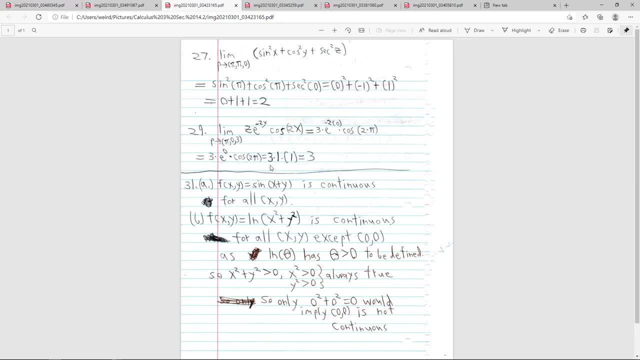 So that's 3 times e to the 0 times cosine 2pi. It's equal to 3 times 1 times 1, which is equal to 3, because e to the 0 is 1, and cosine of 2pi is 1.. 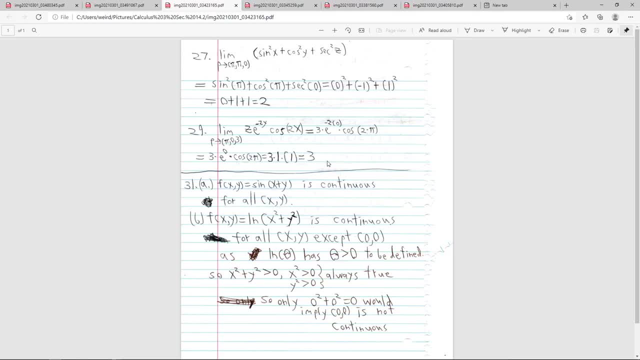 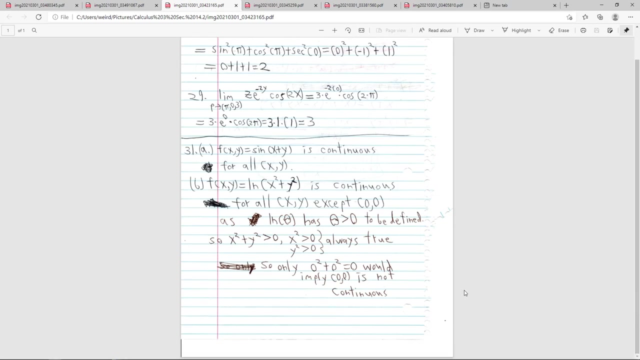 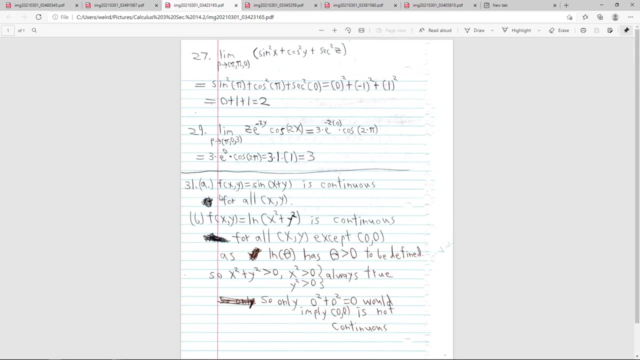 Yeah, Cosine of zero is 1,, cosine of pi is negative 1, and cosine of 2pi is 1, and it goes on, As you know the cyclical nature of it. So now we just do a couple continuity problems. 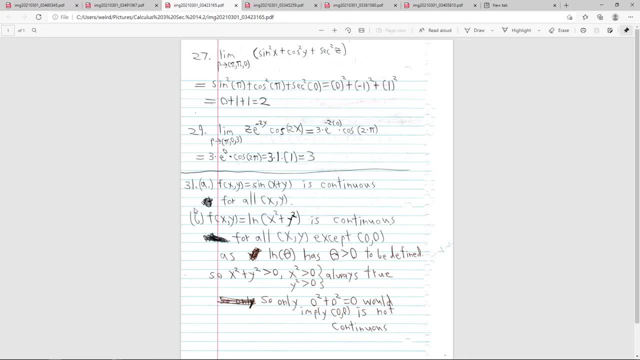 That's it for this section. So f of x- y equals 3.. Yeah, Sine of x plus y is continuous for all x and y. I'm just going to state what these functions are continuous for and show the work accompanying. 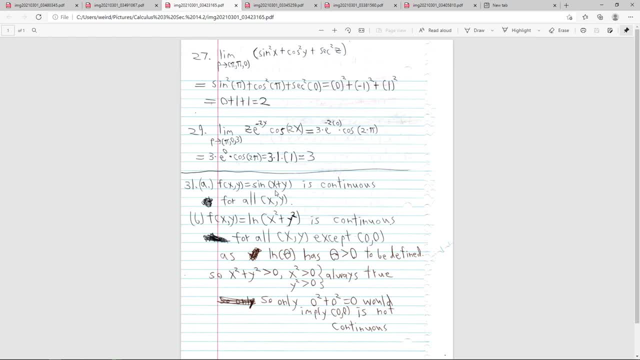 it. So this one- I think that's pretty obvious- Sine of x plus y will be always continuous because the sine function accepts any input value, pretty much. It only has a small range, a narrow range of values. it can take on between 1 and negative. 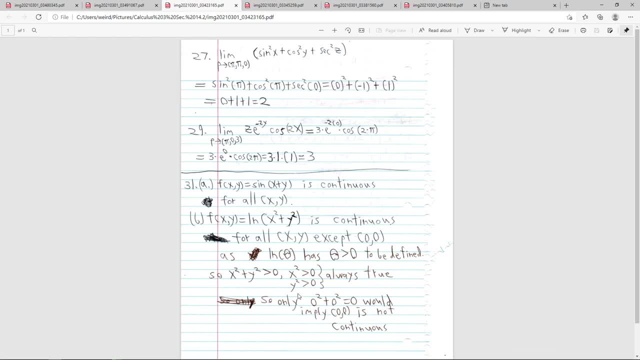 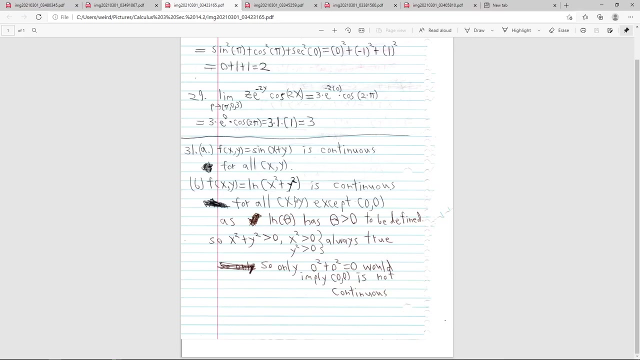 1. But it's domain is all numbers, pretty much as we can tell, At the very least, real numbers, all real numbers. Now, another type is f of x- y equals ln of x squared plus y squared, So ln of x squared plus y squared. 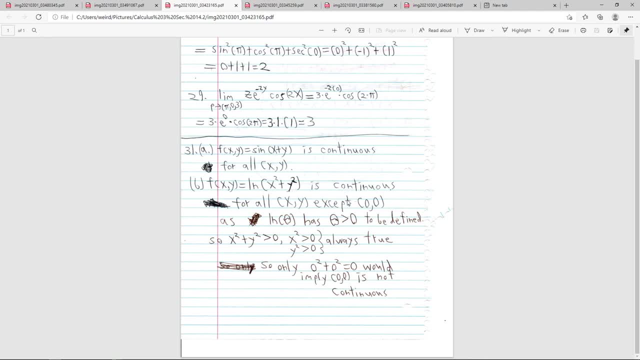 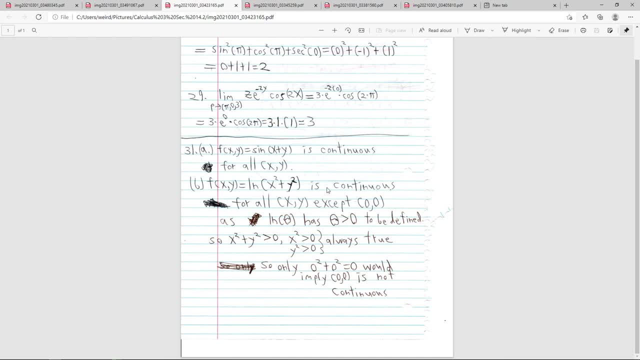 as a general rule. That's why you find out exactly. you know it's except 0, 0 in this case Because naturally there's basically an ln theta, the natural log function basically of any value. You have to have theta. 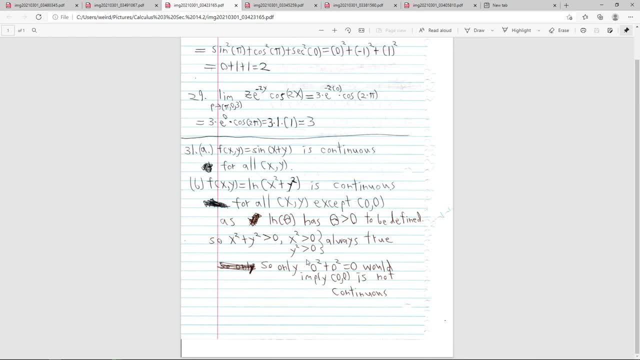 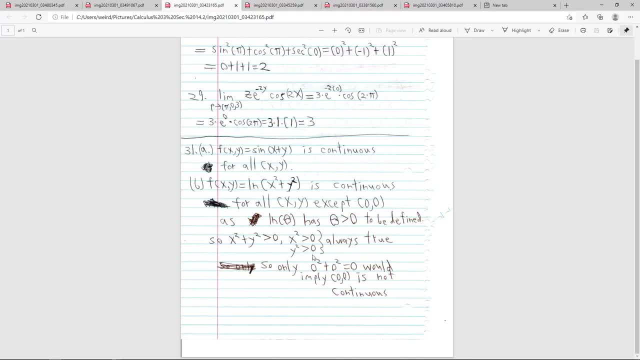 Or greater than or equal to zero Should be the proper thing, But regardless. the point is that these are always positive numbers. The only zero is greater than or equal to zero would imply 0,. 0 is not continuous. That's pretty much what's going on. 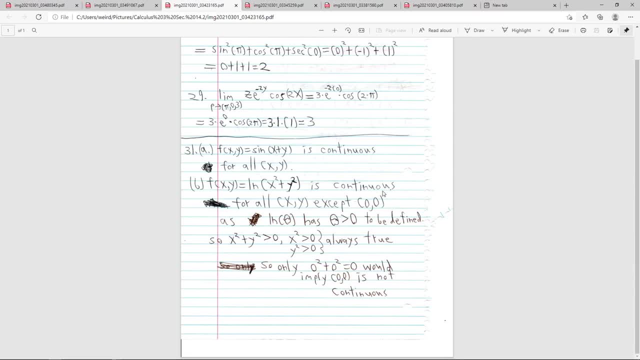 That's the only point. 1.00 would be where it would not be, Because any negative values or positive values that are not, you know, positive values, values except for 0. Like negative 2, if you're squaring negative 2, it's 4.. And 2. 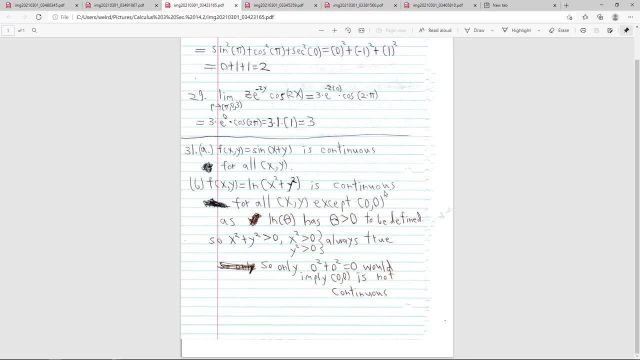 squared is 4.. So really you only have 0 and 0. The only times where you get 0, as the whole x squared plus y squared equals 0, only when both are 0.. Plus x and y are 0.. 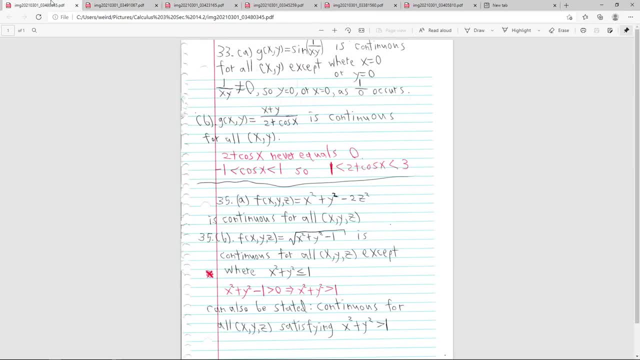 Couple more G of x by y equals sine of 1 divided x by y. This is continuous for all xy, except where x equals 0, or y equals 0. Either one of them- pretty obvious 1 divided by 0 occurring- is not good. you avoid it, or else it will be non continuous. So that exists. 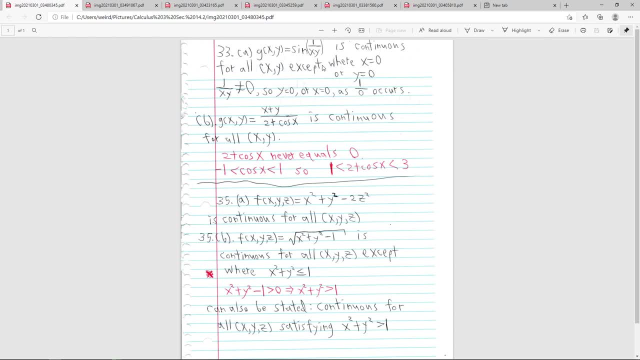 for whenever x or y, because it's a multiplication of them. so anything multiplied by 0 is a non continuous is 0.. g of xy equals x plus y divided by 2 plus cosine x is continuous for all xy. And to demonstrate this, 2 plus cosine x never equals 0.. That expression will never, Because 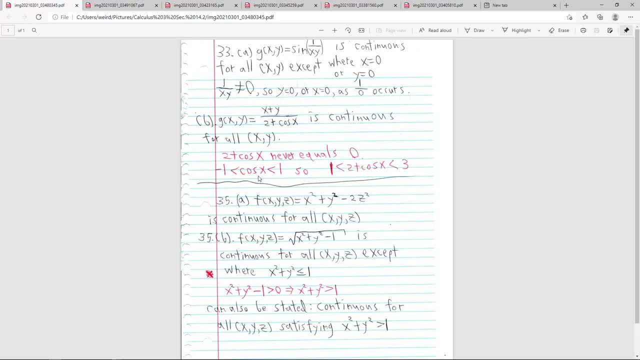 negative 1 less than cosine x, less than 1, that's what cosine x can equal. That's the range, So 2 plus cosine x. you add 2 to each side, You add 2 to that to cosine x and you add 2 to negative 1. 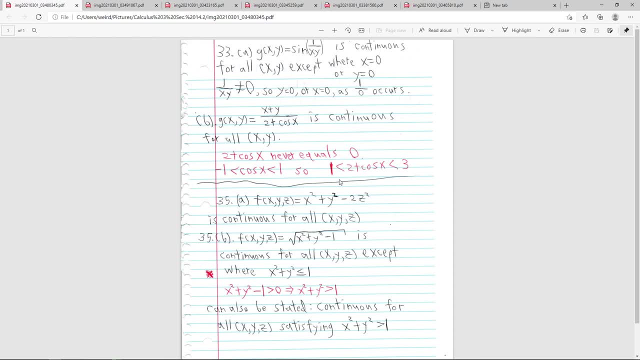 and 2 to 1.. So it could assume any value denominator could be 1 and 3, anywhere between 1 and 3. And that should be less than I keep on forgetting these equal signs. Point is, though, you know, it has to be either 1, it can be greater than or equal to 1, or less than or equal to 3.. 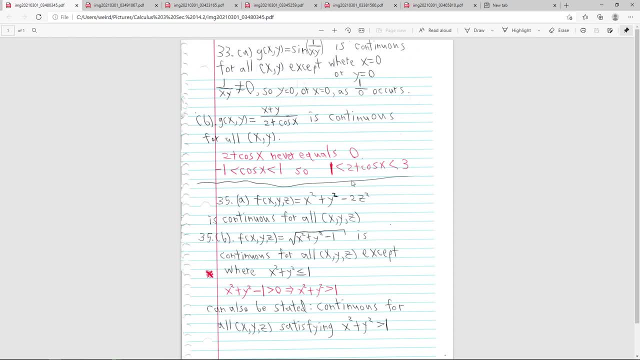 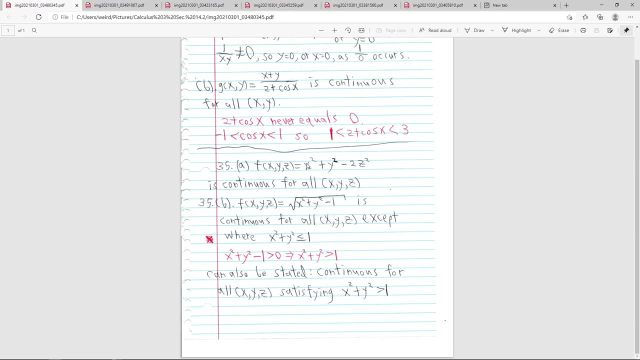 But it can't be anything beyond those parameters. A few more f of xyz equals x squared plus y squared minus 2z. cubed is continuous for all xyz. It's simple. There's nothing That can make it undefined or anything else. A function being undefined is like the number one. 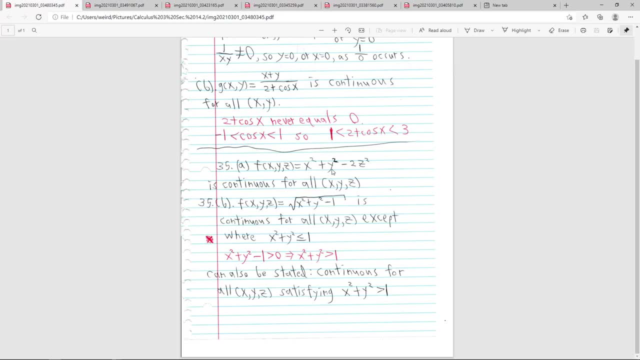 cause of non-continuity. if there's a point where it is not. I think in general That's what we've been looking for, at least to be able to tell right away. So now we have the square root of x squared plus y squared minus 1.. For some reason it's given in xyz when it's just x and y as well. 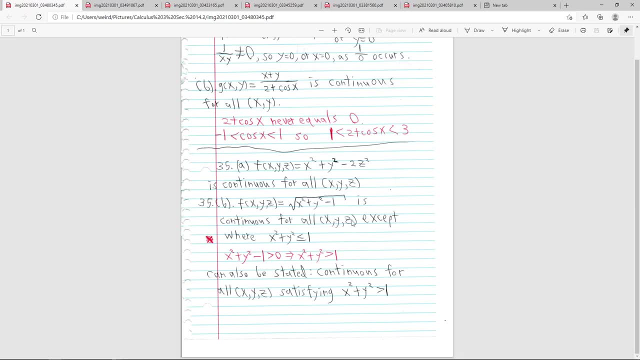 as I can tell, It's continuous for all xyz, except where x squared plus y squared is less than equal to 1.. It's continuous for all xyz satisfying x squared plus y squared greater than 1.. Basically, x squared plus y squared have to be greater than 1.. 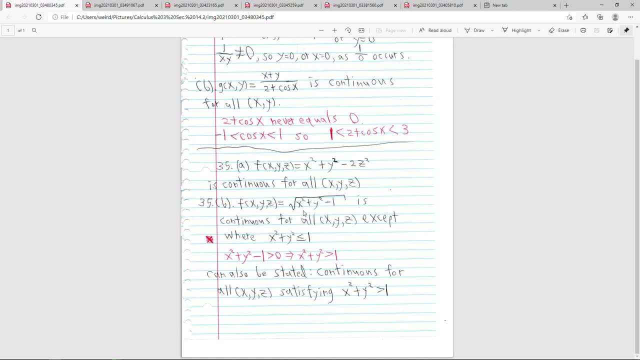 Because x squared plus y squared minus 1 is a square root. So this whole thing has to be: you can't take the square root of a negative number. Yeah, No, you can't, Even though greater than it should be, greater than whatever, Inequalities aside, being a little. 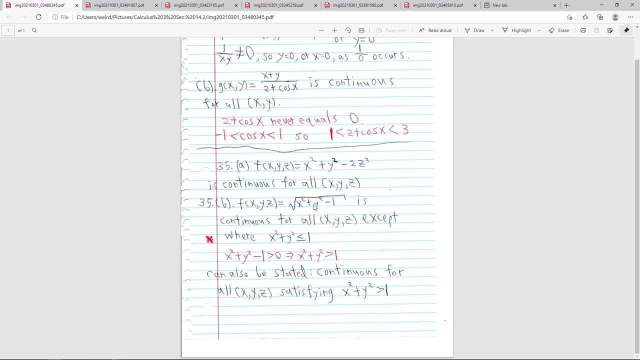 bit off Point is: you get. I think you get the point. So this can be zero. You can have a square root of zero. The square root of zero is zero. It's defined So if x squared plus y squared does. 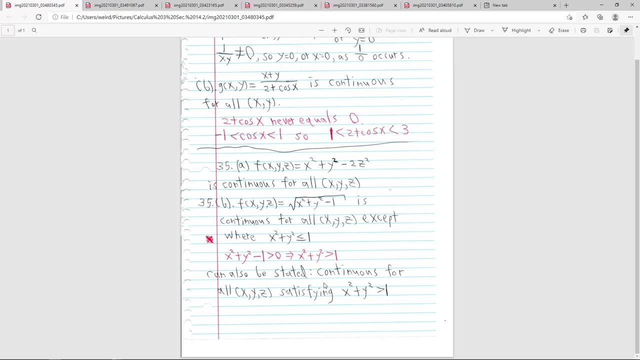 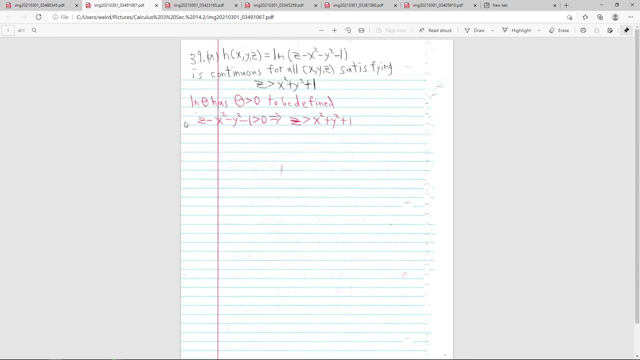 equal 1, then 1 minus 1 is 0 and it's fine. So x squared plus y squared has to be greater than or equal to 1.. Little typo there, but whatever Weird mistake, H of xyz equals natural log of z minus x squared minus y squared minus 1.. And I'm just ending with. 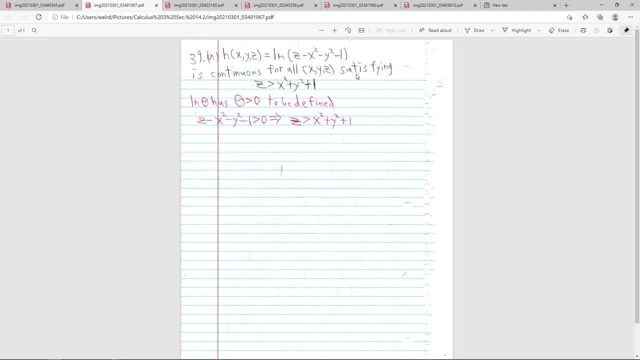 this one. It's continuous for all xyz satisfying z greater than x squared plus y squared plus 1.. Reason is is that you know you have to have your natural log has to be greater than zero, So you just add on each. you add all these terms on the right side. 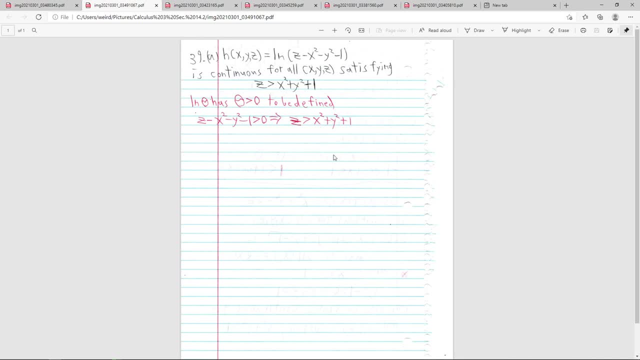 it's greater than zero, And you get z greater than x squared plus y squared plus 1.. That's the way of writing out this thing. So yeah, that's basically all you have to do, So.